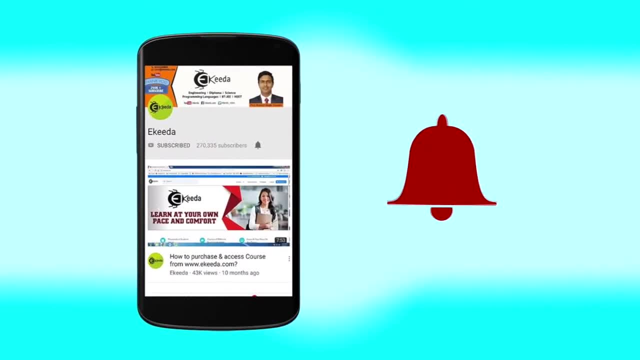 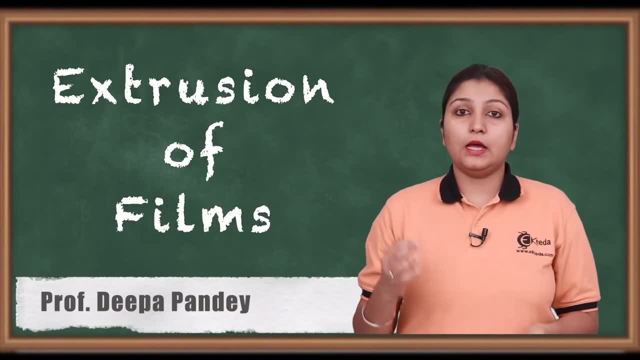 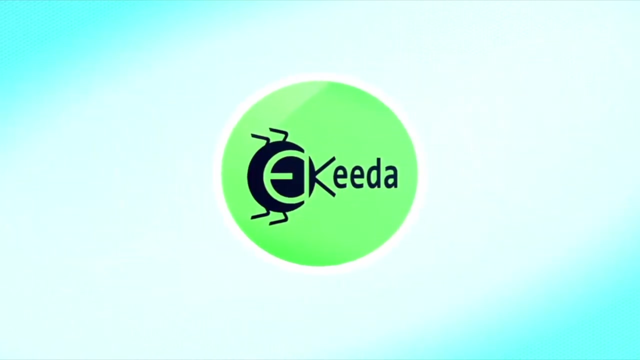 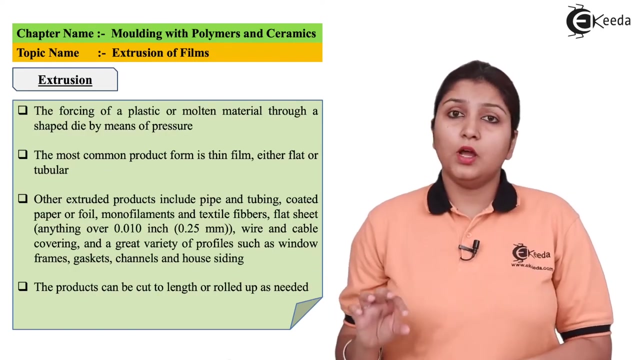 Hello friends, today we are going to see a different method of producing thin plastic other than laminates, which is films, And we can see how the films are extruded by the process of extrusion. So in this diagram you can see this is a normal extrusion process in which a hollow pipe 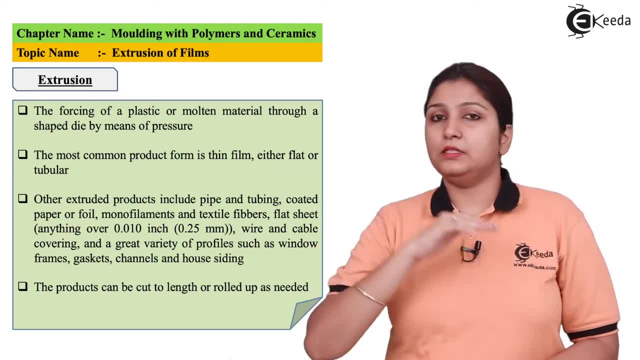 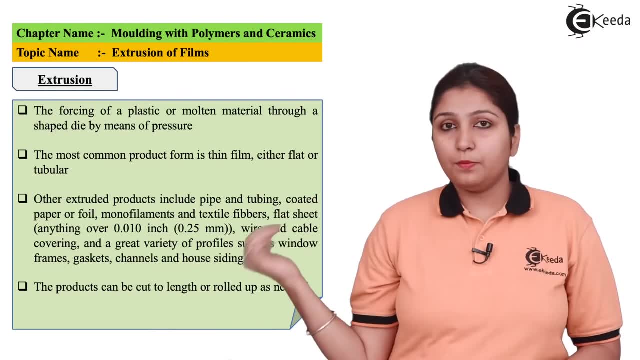 or a circular pipe can be made by easily passing it through and doing the process of extrusion and finally the sheets or the pipes are cut off. How the pipes are made, The same way your sheets can be made. It is a normal extrusion process. So in this diagram you can see how the films are. 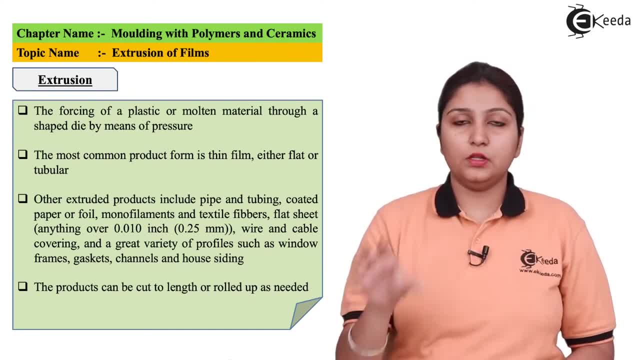 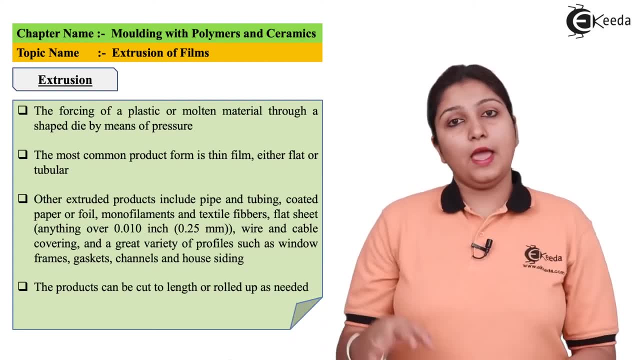 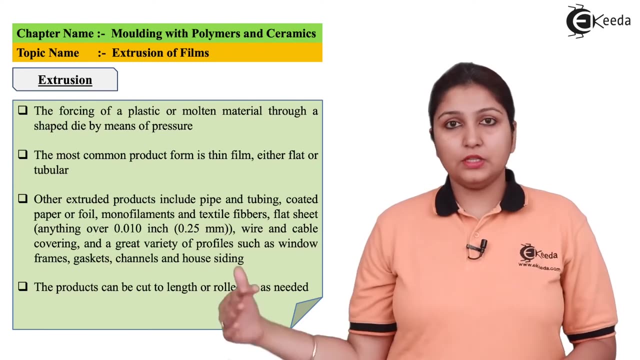 passed through the hopper to your extrusion vessel where it is melted, and it can be passed through a die opening which is in the shape of a sheet, and finally the sheet comes out from the die How? By the process of extrusion, and it is reaching the end and it is getting cut off. So 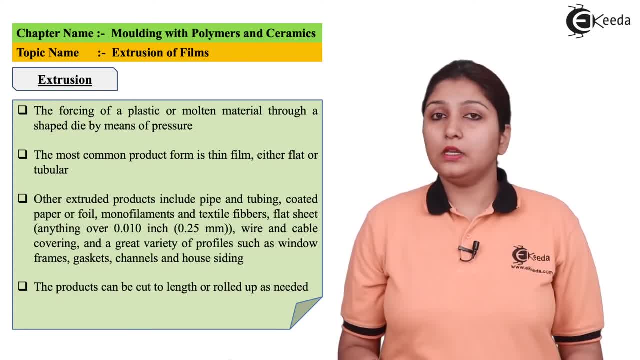 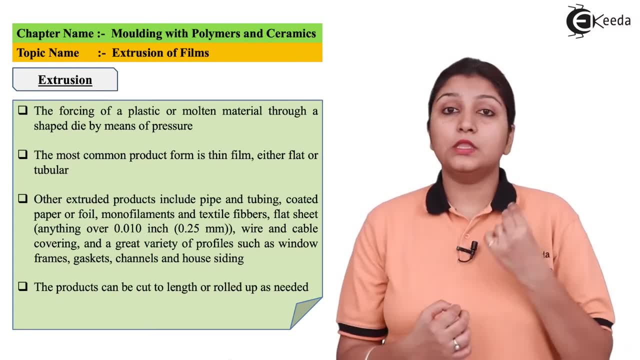 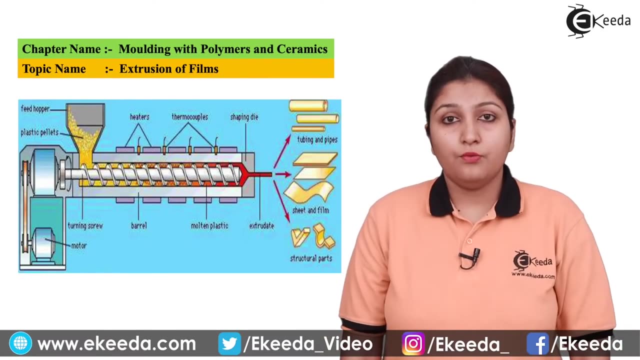 this is the basic extrusion process which can be done either for pipes or for sheets. So extrusion of films can be done to obtain Very thin product which is a film. So in this diagram it is clearly seen how the process takes place. Firstly, there is a hopper through which the material is being fed. Basically, what we do is we. 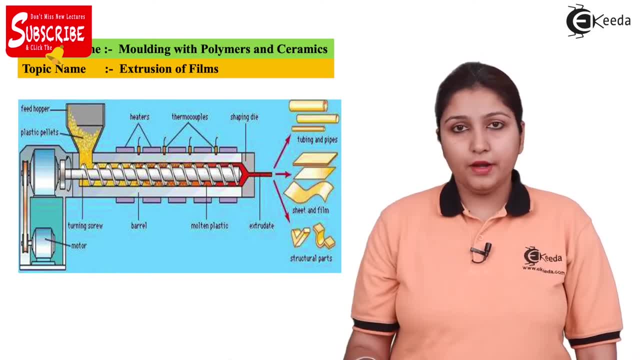 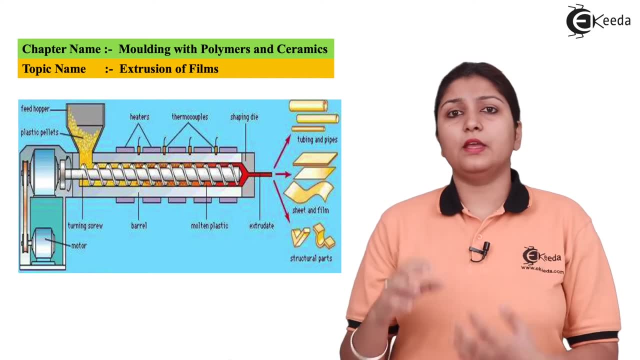 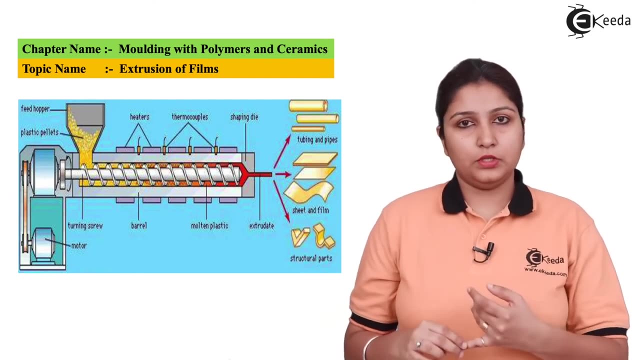 fed thermoplastic matter. So it is getting fed again, it is getting melted inside your extrusion box where your exact melting is done and it is getting liquefied. Then the third stage come: it is getting extruded. You can do any of the process, like you can do the injection process, or you can do 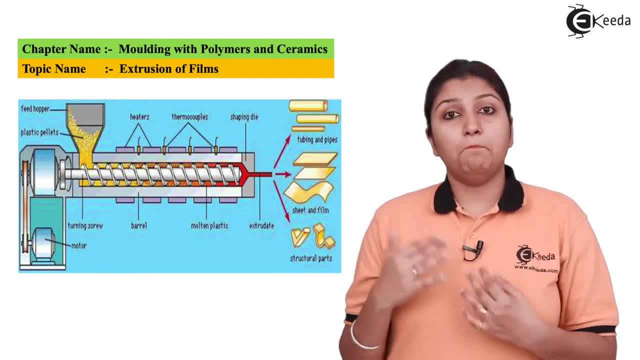 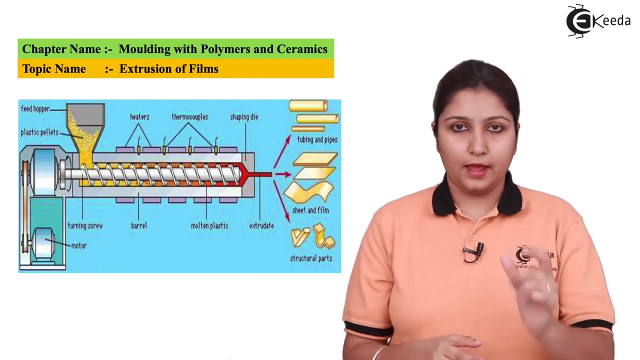 the screw type extrusion process. Anything can be done, but the final aim is the product should get extruded out through the die. So the die would be having the shape either of a pipe either of a sheet. that you can see. the type can make different products, The easily shape you can give to the die. 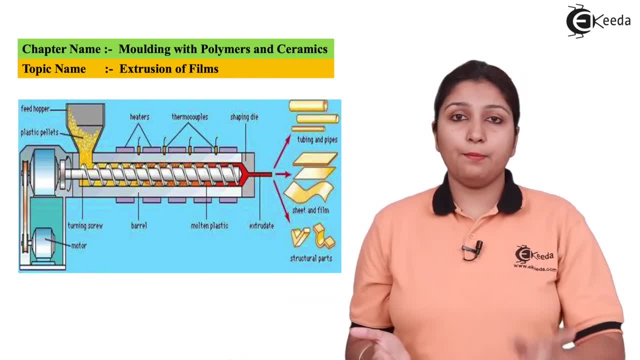 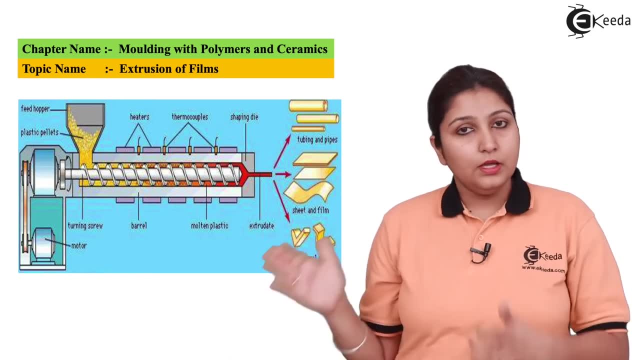 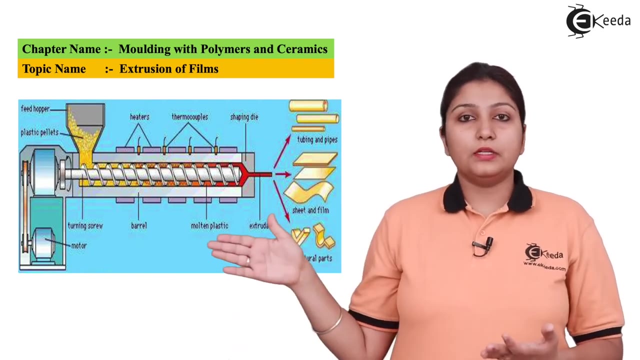 So the product is coming out, but the product is having the shape of the die, which is being kept. If it is a sheet, you can get a sheet, If you can get a pipe. The product is coming out, then it is cutted or slitted according to the need, but this is done only after the product gets out. 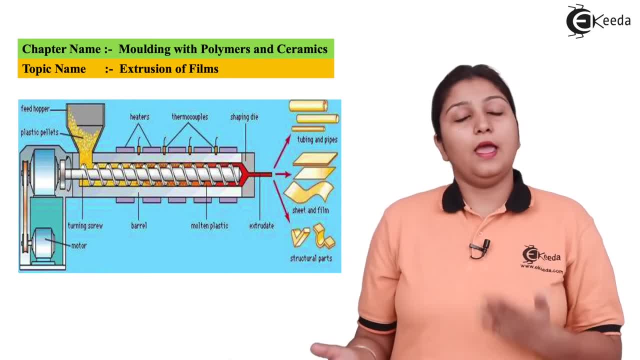 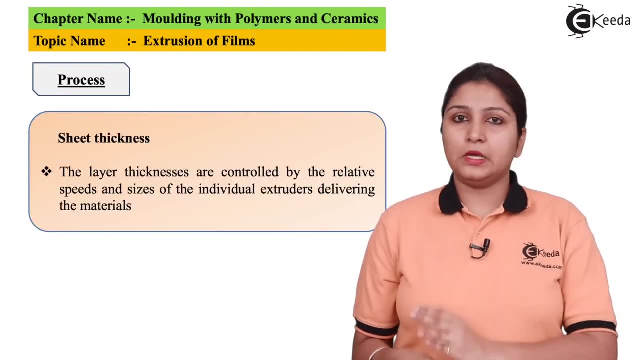 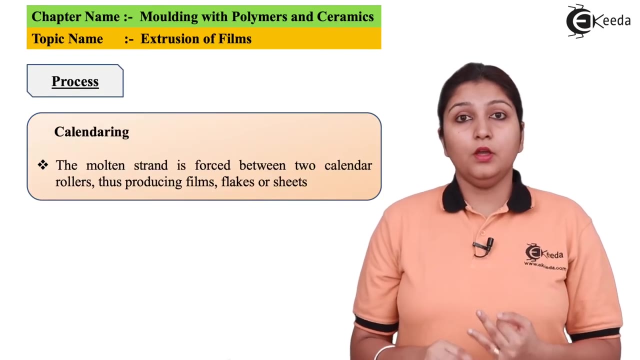 So slitting can be done after the product is made, and then this is cooled and then, finally, it can be used, as it is using In filmmaking, three things you have to keep in mind: One is your sheet thickness. Second, how cooling is done. and third, your exact calendaring process. 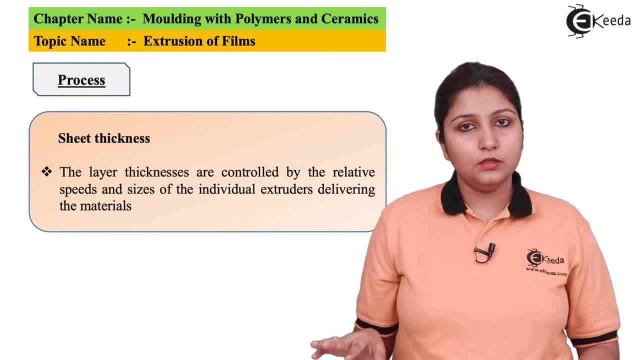 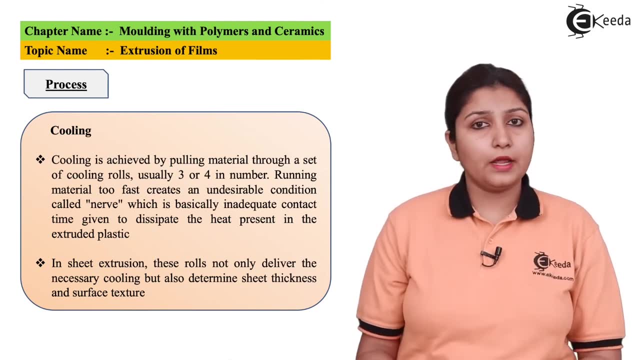 So sheet thickness can be controlled by controlling your die size. Cooling can be done by providing external rollers, which gives you a cooling action, or it can be in the form of air type, or it can be either in the form of water type. And last is your calendaring process. 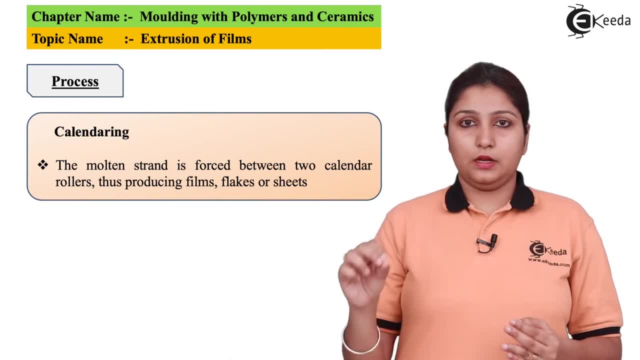 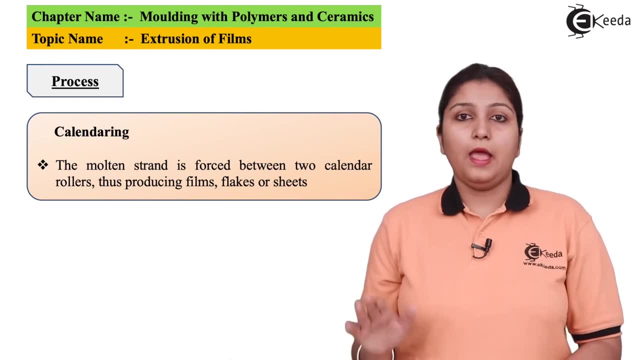 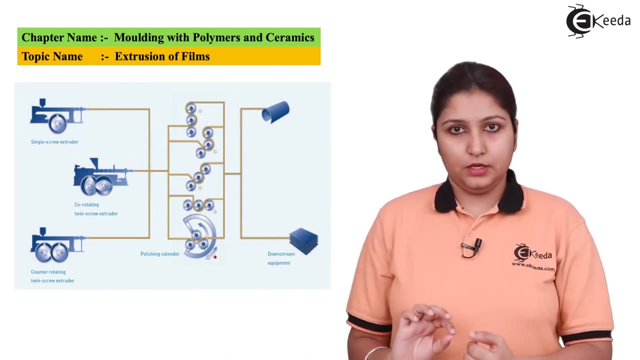 This is done only when you need very less thickness of sheets or films. So two or more rollers can be used to just reduce the thickness of your film and it can be passed through. So in this diagram you can see there are three type of extruders at the starting stage. 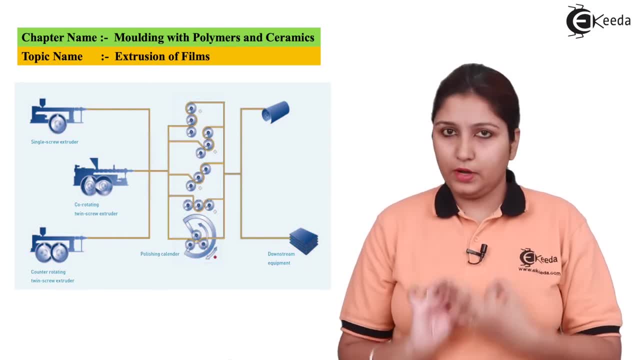 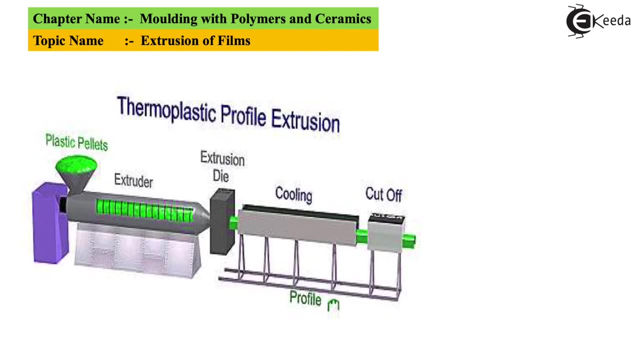 One is your single, second is your core and third is your counter extruder, So your material can come through all these extruders. In between you can see your exact calendaring process where you have different types of rollers through which your material passes. 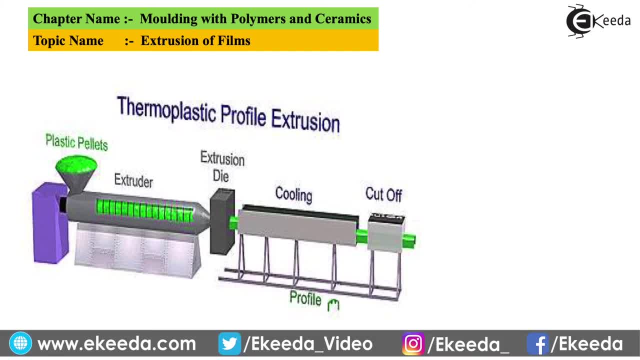 And in the end you have finishing calendaring rollers. So in this way, your tube is coming or your film. The film is coming, which is getting calendared, that is, the thickness is getting reduced And finally, it is reaching the end where it can be cut off, but the desired shape can be obtained. 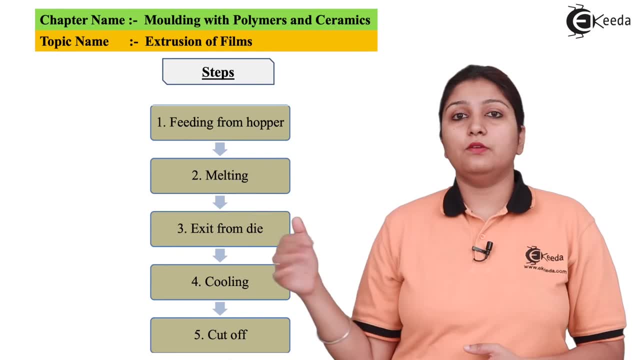 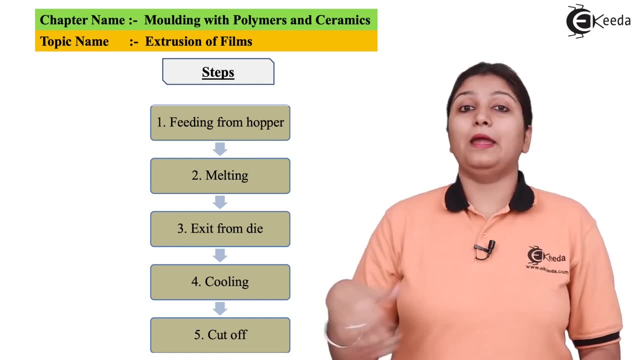 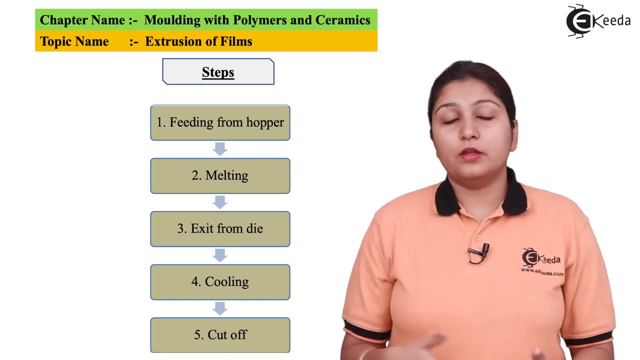 But this is done for sheets. So sheets can be in the form of plain single sheets. You can cut off that, silt it off and use. Secondly, you can keep a roller where piled up sheets can be collected. So both the ways the sheets can be collected, but it has to get cooled for getting it used. 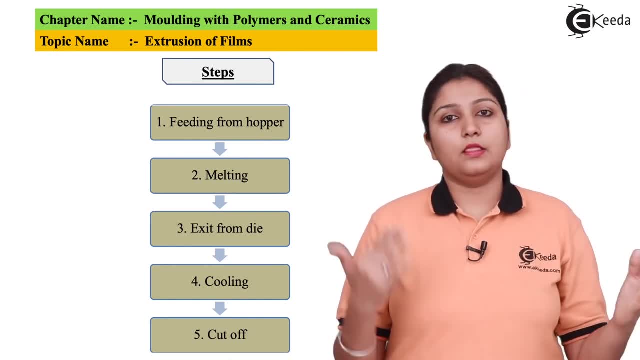 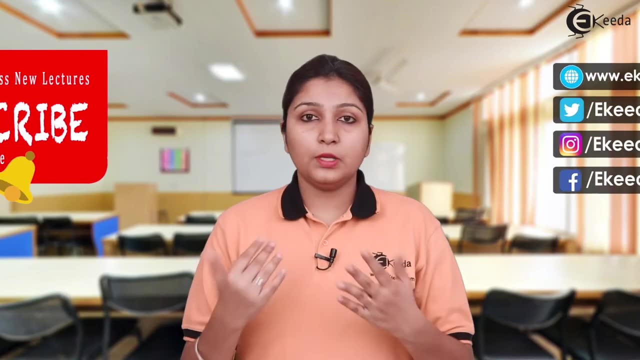 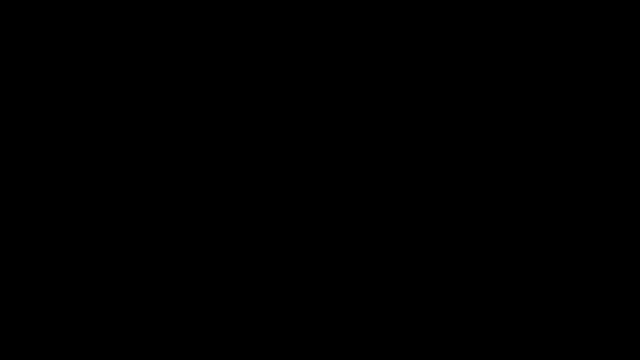 Or for a useful purpose, and then silted, and then again, the things can be done, but according to the use. Thank you for watching this video. Stay tuned with eKIDA and do subscribe our channel. eKIDA. Subtitles by the Amaraorg community.